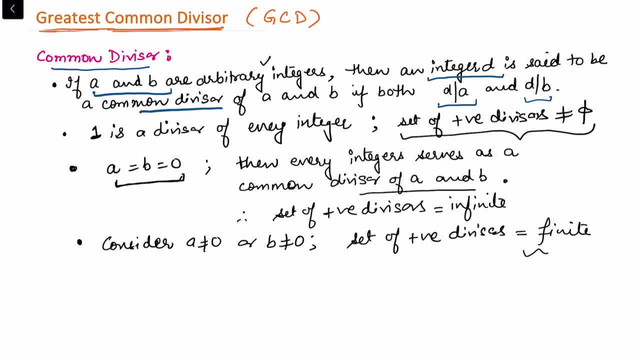 So here I write: set of positive divisor is finite, and as the set is finite, so we can find the greatest common divisor in that set. So now we are ready to define the definition of the greatest common divisor. It says: let a and b be given integers and with at least. 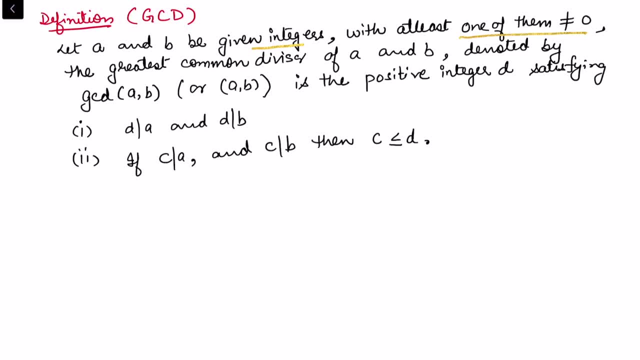 one integer, So let a and b be given integers. and with at least one integer, So let a and b be given integers. and with at least one integer, So let a and b be given integers, and with at least one of them, is not equal to 0.. The greatest common divisor of a and b, denoted by gcd of a and b or. 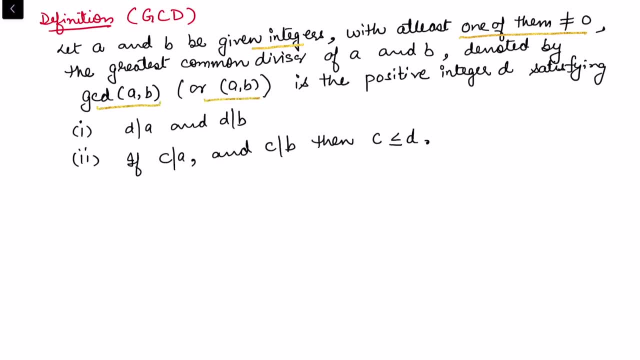 we can simply write down into the parenthesis: a, b is a positive integer d. So greatest common divisor is a positive integer d which satisfy these two property. Since it has to be greatest common, so it is common, so it divides the, both the integer, and also it is greatest So for any. 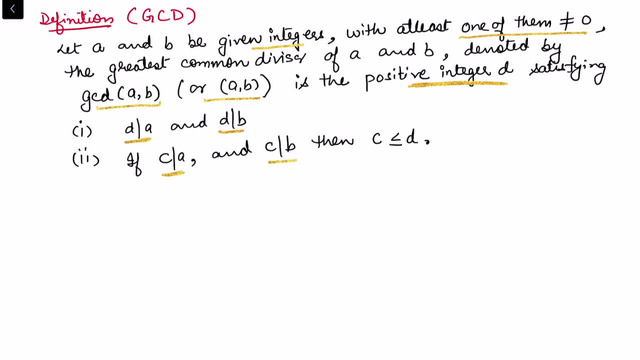 other divisor say: we consider c divide a and c divide b, then c must always be less than or equal to d, So n if the d satisfy d, so it is a positive integer. So let a and b be given integers, and with: 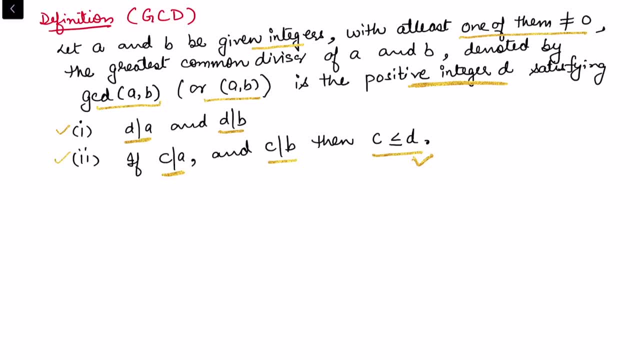 these two condition. then we consider that d is the greatest common divisor of a and b. We now consider some example. Let us say we want to write down the greatest common divisor of minus 12 and 30 and to write down the greatest common divisor, I first need to know what are. 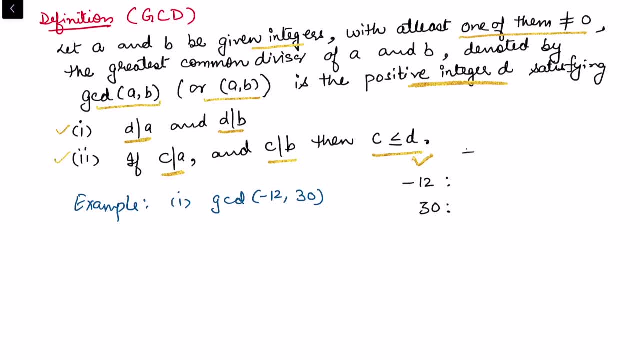 the divisors of these number. So let us only write down the positive divisors here. So when I write the positive divisors for 12, this is 1,, 2,, 3,, 4,, 6 and 12- and for 30,. 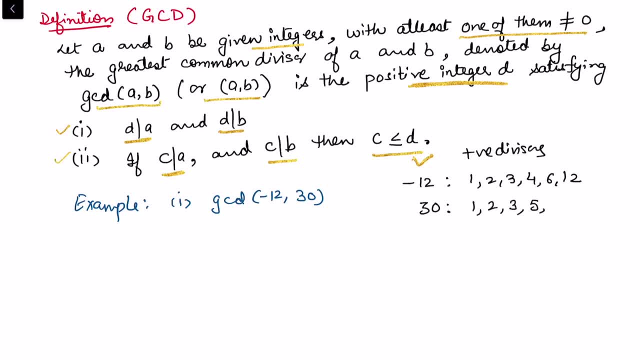 the positive divisors are 1,, 2,, 3,, 5,, 6,, 10,, 15 and 30, and you can see that among the positive divisor, the common divisor, which is the greatest, is 6.. So we can simply say that the gcd of minus 12 and 30 is 6, because this 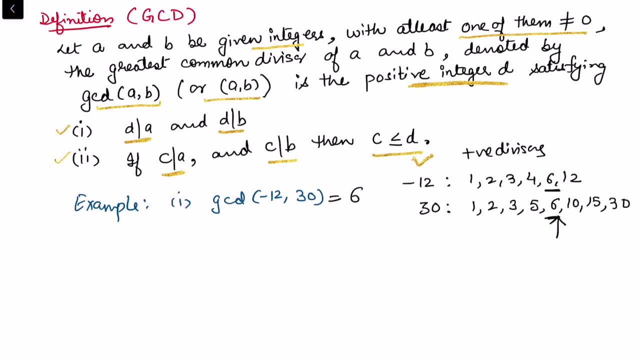 is the highest common divisor. There are other common divisors also, as we can see that 1,, 2,, 3 is appearing here also. 1,, 2,, 3 is appearing here also and 6 is also in the common. So 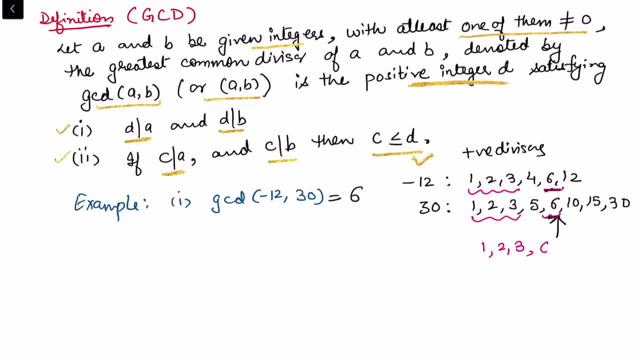 if I want to write down the common divisor, this is 1,, 2,, 3 and 6.. These are the common divisors and among this this was the highest or this was the greatest, So it becomes a gcd. In the another example we can see that if I want to write the gcd of 8 and 17,. you. 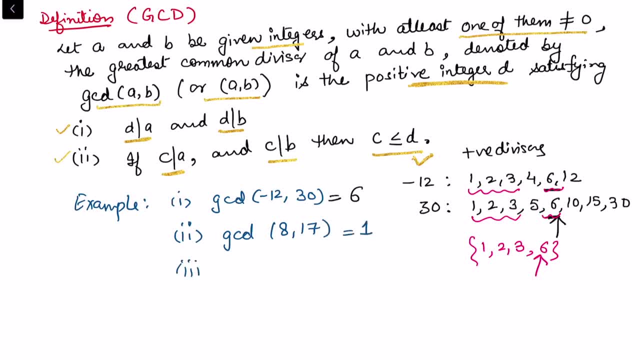 can see that greatest common divisor is 1 and in similarly, one more example I can consider greatest common divisor of minus 5 and 5.. So here you can see that greatest common divisor is 5, and we note that it is always possible to write the greatest common divisor. 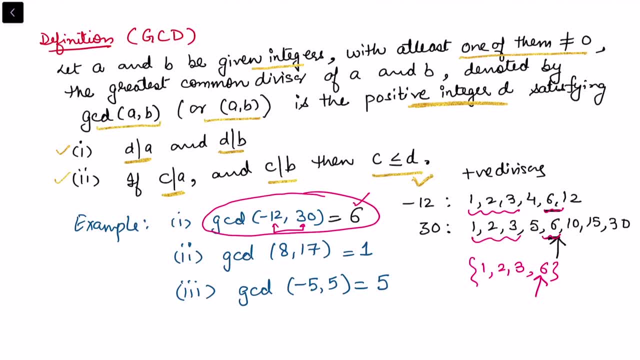 as linear combination of the integers. So for in this case, suppose we write the greatest common divisor, gcd, of minus 12 and 30, which is written as 6.. So I want to write as a linear combination of minus 12 and 30.. These are the two integers, So I can multiply 30. 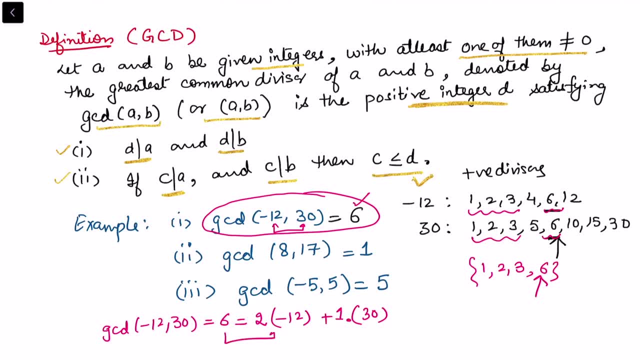 by 1 and by 2.. So you can see that this satisfy the equation. So it is possible to find out these two integers that I have written here, 2 and 1.. So now I will write down the theorem. 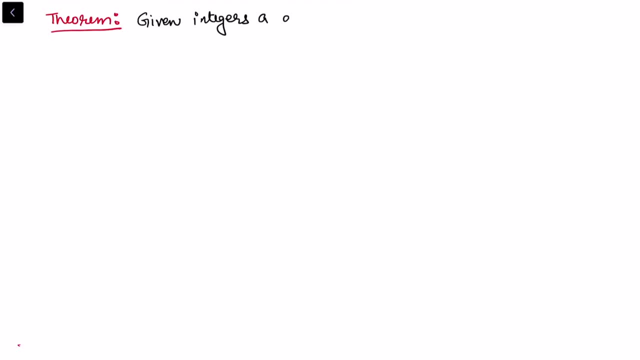 which explain this result. So the theorem says: given integers a and b and not both of them are 0. So that we can find The greatest common divisor. So we write not, both of which are 0. So in that case, 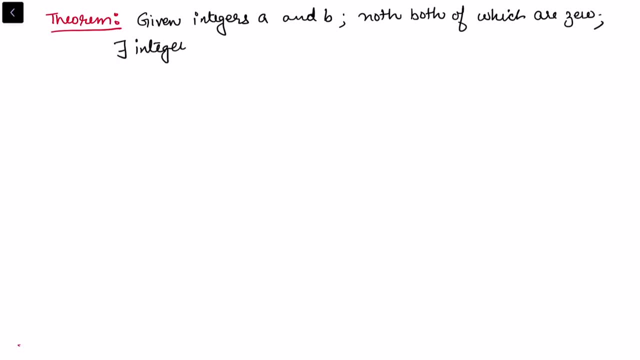 there exist integers x and y, such that we can write greatest common divisor of the integers a and b as a linear combination, ax plus by. So now to prove this theorem, I will consider a set. So considering the set of all positive linear combination of a and b. 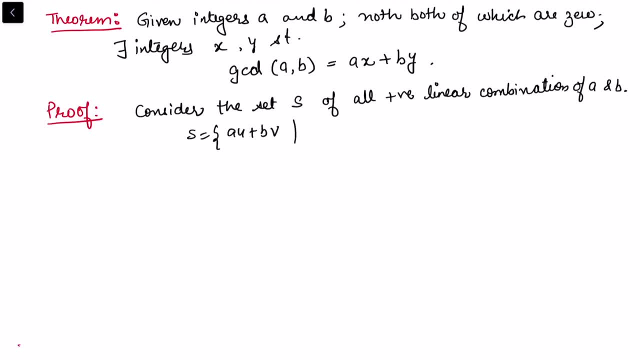 So suf is equal to au plus bv, such that au plus b times v is greater than 0 and uV belongs to integer. So we say that this set s is non-empty. So this is what we first need to notice down. So we write down here, noting that s is non-empty and to prove that this: 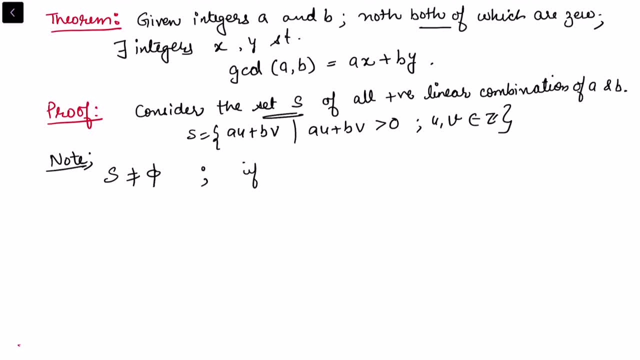 is non-empty. we can simply consider that, as we have said, not, both of which are 0. So let us consider that if a is not equal to 0. So we can write this integer absolute value of a equal to a times u plus b into 0, and this belong to s. so initially, if a is equal to minus 1, then 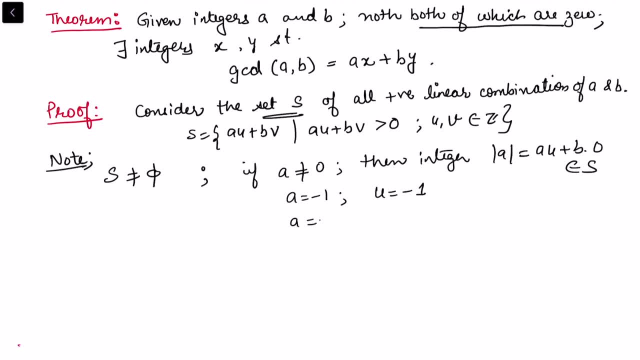 we can consider u also equal to minus 1. if a is equal to plus 1, then we can consider u is equal to 1. so for this choice of a, whenever this is non-negative, and depending upon whether it is minus 1 or plus 1, we can select the corresponding value for u, and hence we can say that absolute. 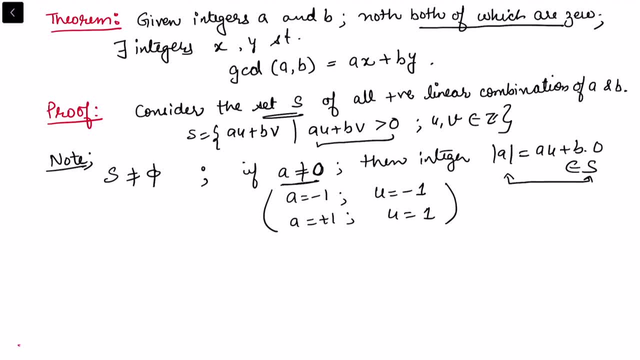 value of a belong to the set s. this satisfy the given condition and we can say that the set is non-empty. now, as the set s is non-empty, and by well ordering principle, we can say that s must contain a smallest element, contain smallest element, and let me to call that smallest element. 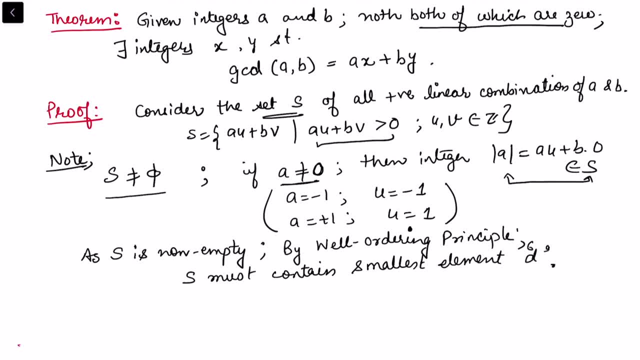 as d. so when i call the smallest element as d, and since we are saying that d belongs to us, it is smallest element in the set d. so d must be of the form some a, x plus b, y, and this x comma y belongs to integer. so this is the representation of d by the. 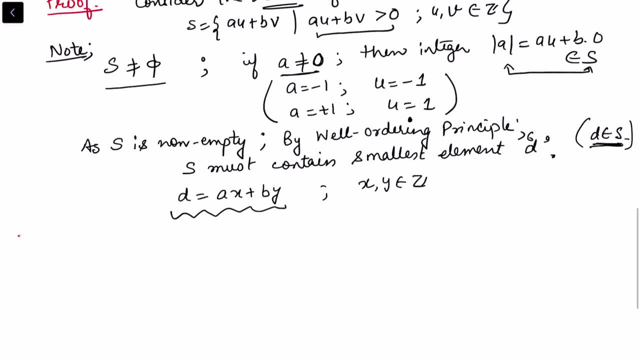 selection of the d as d is the smallest element which belong to this. and what we claim is: we want to claim that d is the gcd of a and b. so if we can show that d is the gcd of a and b, we have already shown that d can be written as a linear combination. and if we can show that d is gcd of 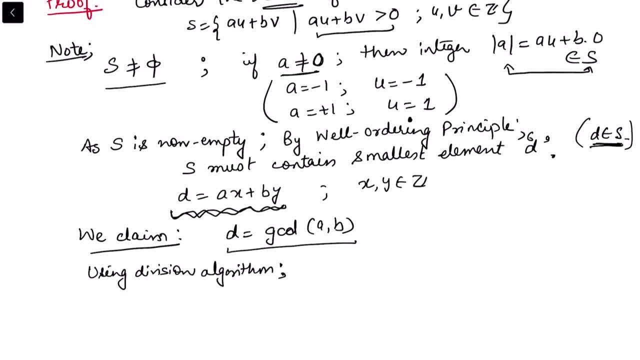 a comma b. that proves our result. so now, as i want to show that d is gcd of a and b, and to show that, i first need to show that d is a common divisor, and for any other divisor this is the largest one. so i am using a division algorithm and in that division algorithm we can always obtain the. 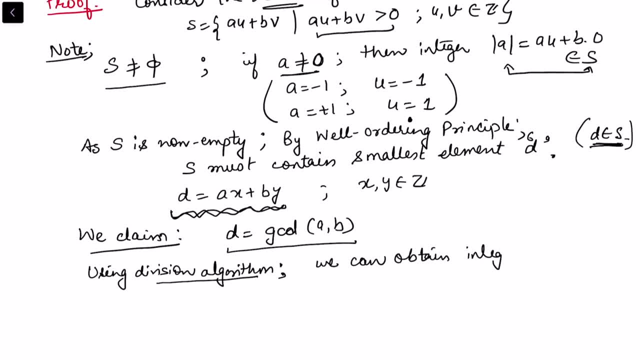 integer q and r. so let us write down: obtain integers q and r such that we can write down that whenever a is divisible by d, so it is written as qd plus r, and since we are dividing a by d, so the remainder have this condition that it is strictly less than d. we have already considered. 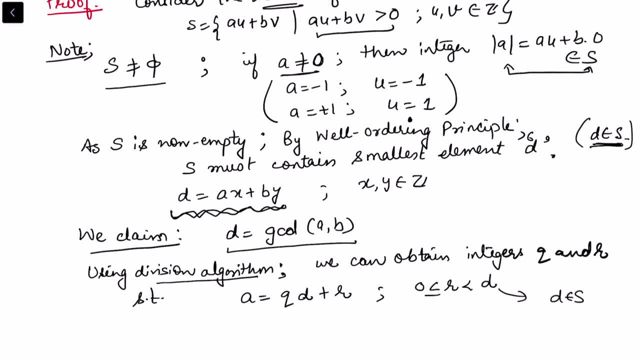 d to be a positive. so we know that d belong to s and s is a set of positive integer. so d is already a positive integer, so we can see that. so here we do not need to put an absolute value while applying the division algorithm. now a is equal to qd plus r, so this: 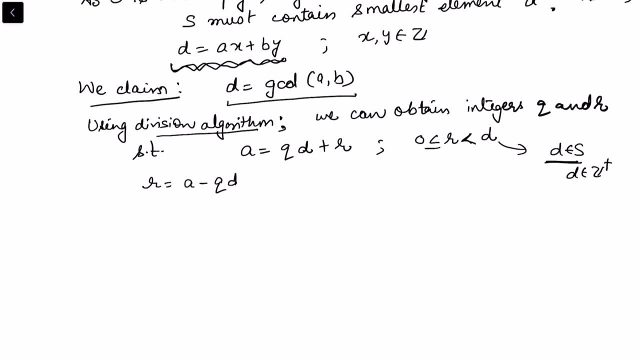 implies this is same as r is equal to a minus q times d and this is same as a minus q times for d. we already have this expression ax plus by. substitute this here. so this is ax plus by, and that becomes a into 1 minus q times, x plus b into minus qy. 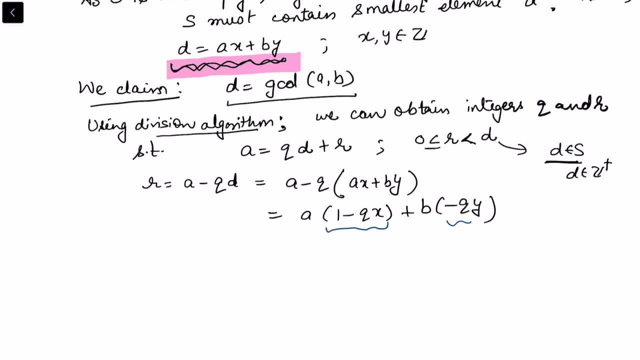 Now noticing that this is a times something and b times something. so if you assume that it is x dash and this is y dash, so what is happening is that we are writing r as a into x dash plus b into y dash, and here we are saying that r is greater than or equal to 0. so if r is strictly positive in that, 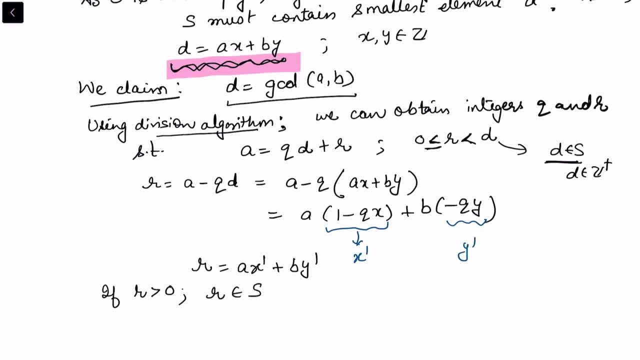 case this implies r belong to the set s because of the representation it have, but this will contradict the choice of d, because we have selected d As the smallest element. so this contradicts choice of d, and we said that r is strictly less than d. so 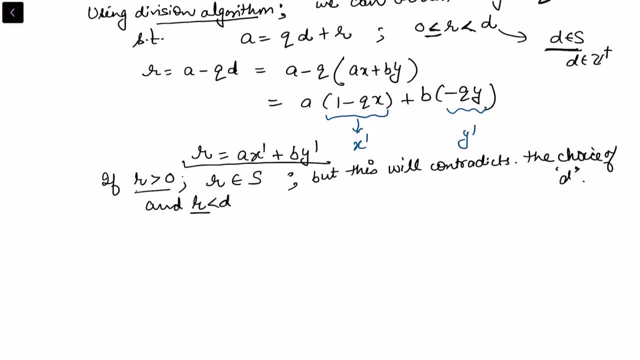 considering these situation in mind, that if r is a strictly positive and it is less than d, this will always contradict this choice. so this implies the only choice we have. this implies r must be equal to 0. so if r is equal to 0, so the our initial selection that a is equal to q into d plus d. so 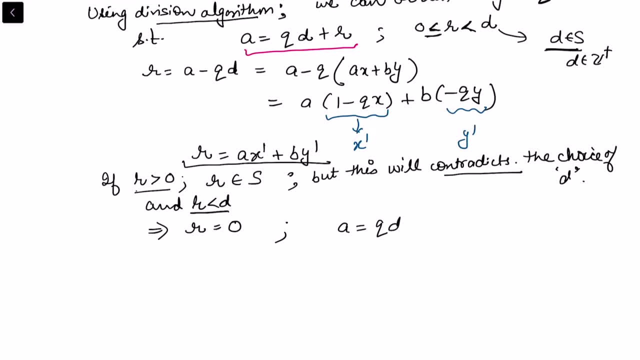 that means we have: a is equal to q times d. so this implies d divides a And in the similar reasoning we can show that. so with similar reasoning we get d divides b. so that shows that d is a common divisor of a and b. so this is a common divisor of a and b now as this: 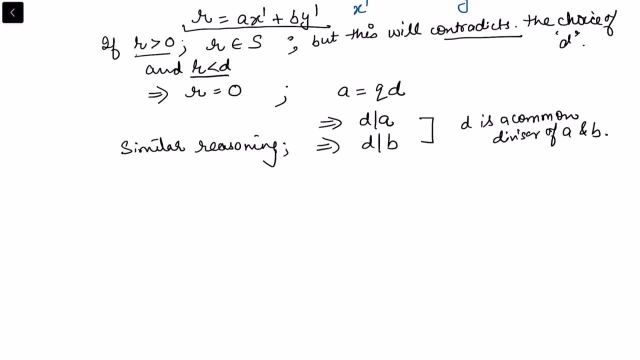 is a common divisor of a and b. so now the first condition of the gcd definition is satisfied, and i now only want to show that if there exist any other divisor, then d is the largest among all. so now, let us choose that. Now, if c is any arbitrary divisor of a and b, then c must divide their linear combination we have 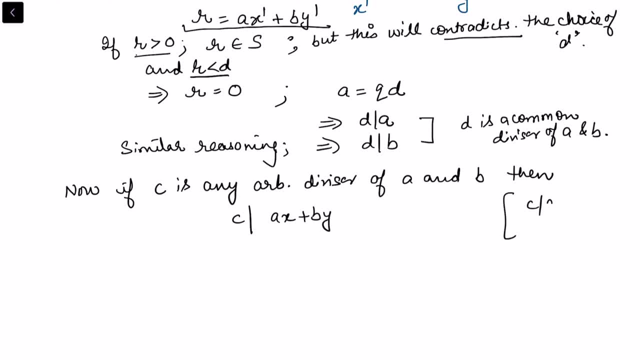 already done this in the basic properties, that whenever c divides a and c divide b, c must divide ax plus by, and this implies c divides d, because we have already used d, same as ax plus by, and so to prove this theorem i must would have considered this as positive divisors, so kindly correct this. 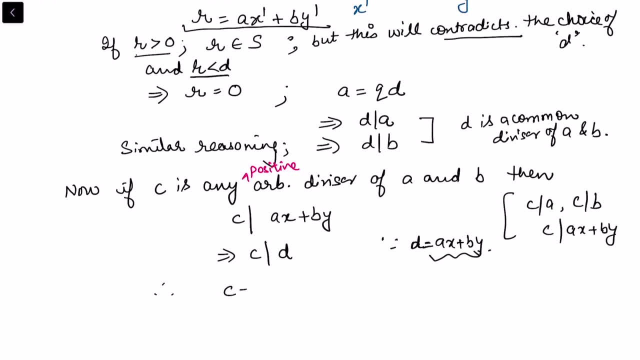 this is a positive divisor and d is also positive divisor. so this means: since c is a positive, so c is same as absolute value of this. this is always less than or equal to absolute value of d, which is equal to d, so hence we can say that d is the gcd of a and b. 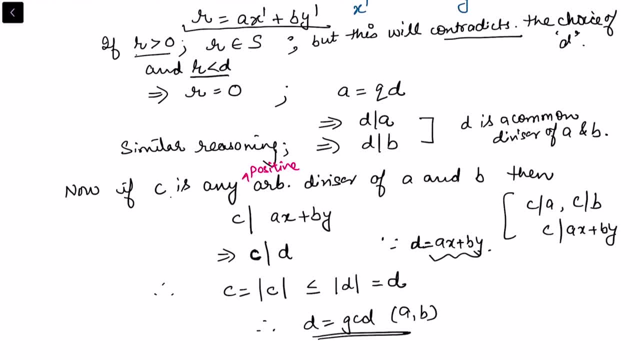 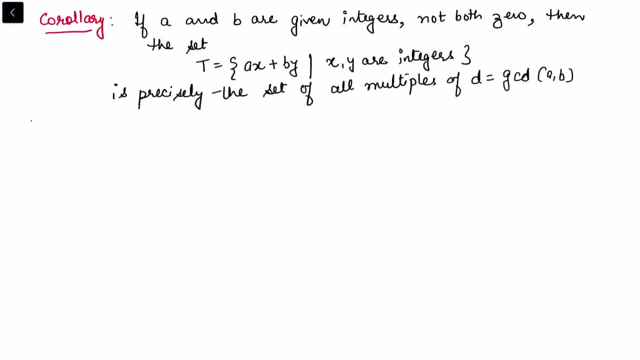 and this satisfies both the condition that for any arbitrary divisor this is the largest among all, as the consequences of the above theorem. now i can immediately get this corollary as that if a and b are given integers, not both 0, then the set t, which is ax plus by, and x and y are integers. this is: 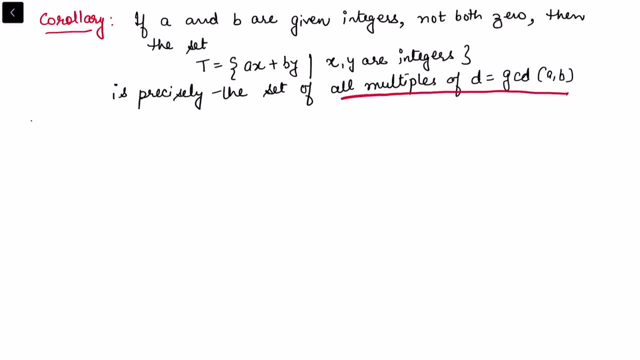 the set of all multiples of d. and to explain this, let me to first consider an example. suppose that we consider two integers- a is equal to 6 and i consider b is equal to 15- and then we consider a set- t, and let us write down this as a linear combination of the two integers that we have. 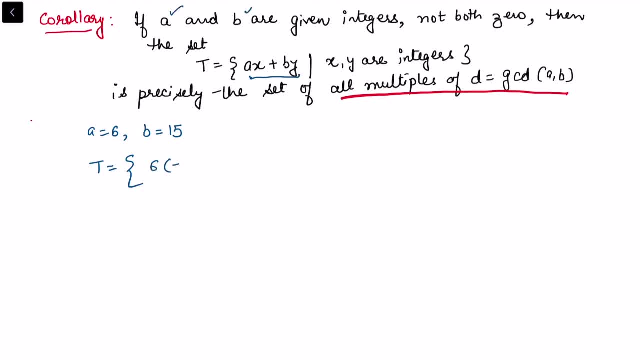 selected a and b. so in this case, let us take combination 6 into minus 2 plus 15 into 1, and then let's take another combination: 6 into minus 1 plus 15 into 1, let's take another combination, and so on, so you can take different combination and if we notice that this is same as this value, 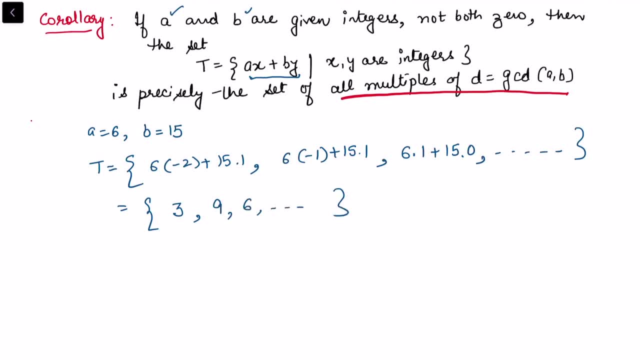 is 3, 9, 6 and so on. and if i see that, what is the gcd of 6 and 15? so you can see that greatest common divisor of 6 and 15 is 3, because 6 has positive divisors, as 1, 2, 3, 6 and 15 have the positive. 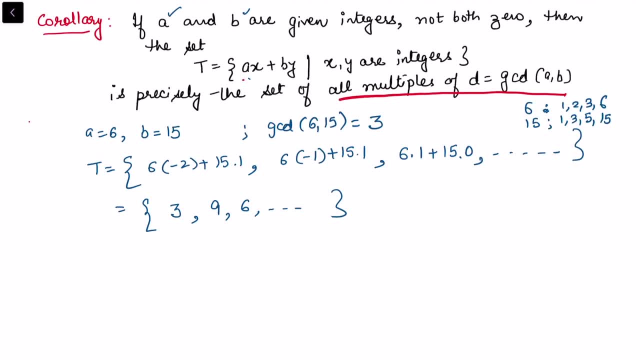 divisors as 1, 3, 5 and 15. note that we have put it a more generalized condition. we have simply: the negative multiples are included in this set. we have not included that ax plus by is strictly positive. but if you include that ax plus by is strictly positive, as we have defined in the 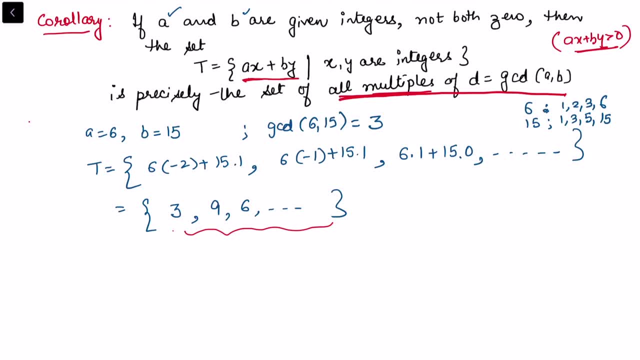 statement of the previous theorem. in that case, here we can see that d act as the smallest element. if not, if this condition is left, if this condition is not included, then we can consider even the negative multiples of the greatest common divisor. now let us do the proof of this corollary and we 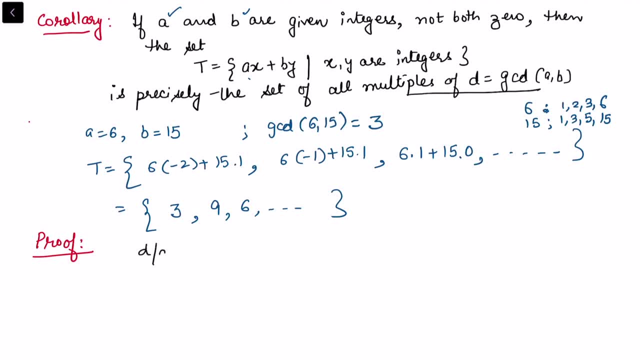